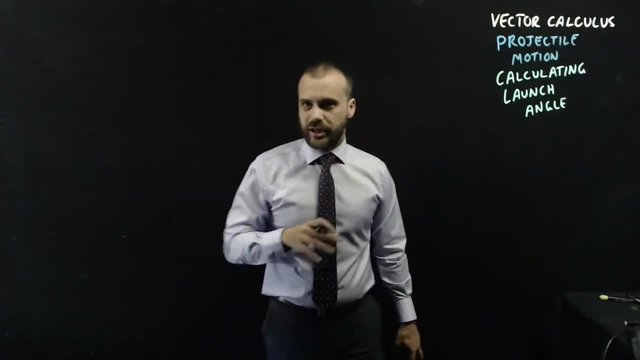 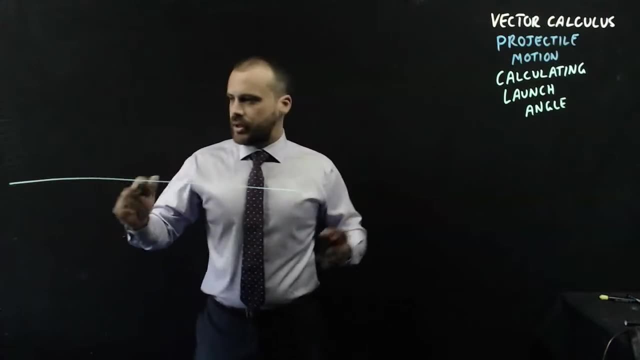 So we're doing projectile motion. This time we're going to calculate the launch angle. So let's just set up a question. Let's put the ground here, right? Okay, so we've got the ground. Let's make like a little tower that's two meters high. 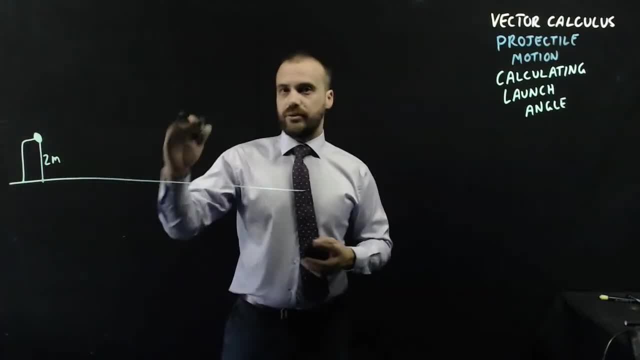 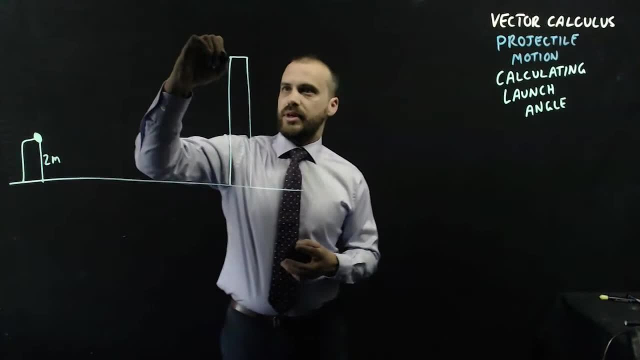 And let's put our particle here and we're going to launch it from there And we're going to launch it up against this wall here. right, There's a target here that we want to hit Now. that target is five meters high. 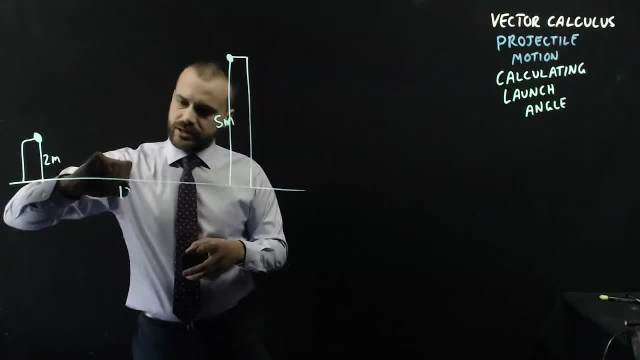 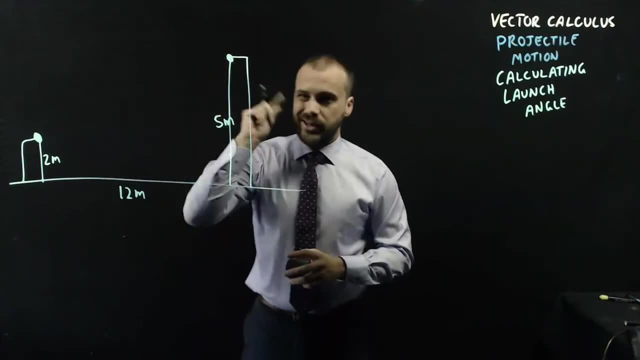 And let's say that the distance from here to here is 12 meters. All right, there's my question, and I want to launch this projectile to hit that Now. if you're a bit of a clever cookie, you might be thinking. 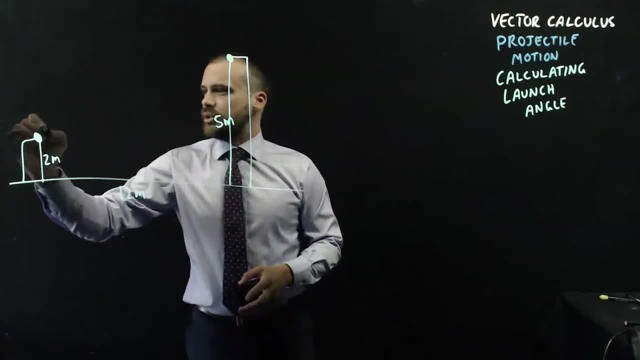 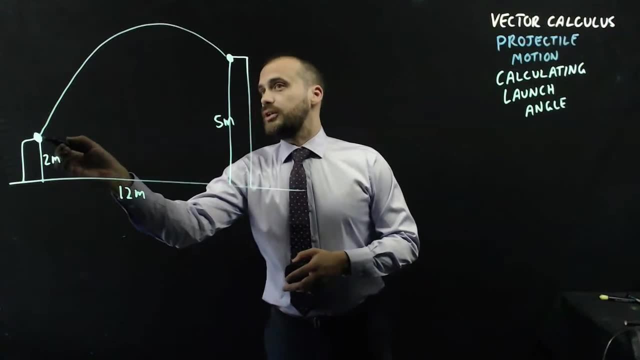 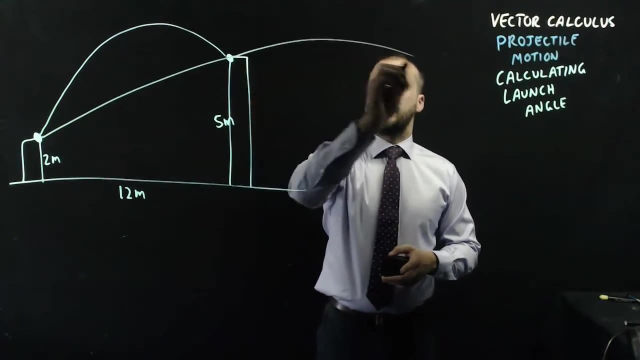 well, hang on. there's two ways I could do this. I could launch it up into the air and down, or I could launch it. I could launch it to get it on the way up and if it was to go past it, it would like start turning over there somewhere. 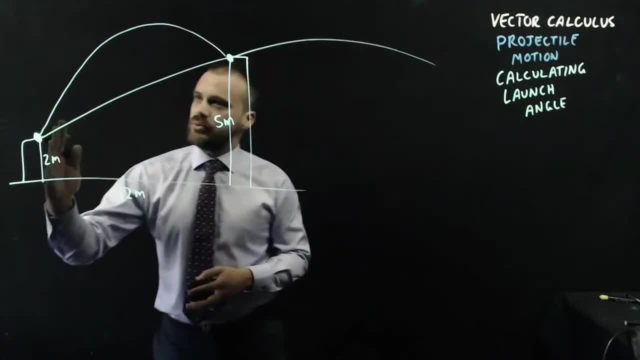 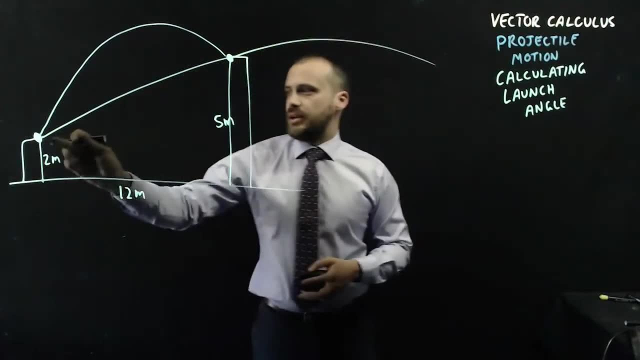 So there's going to be two answers to this question: One where it goes, launches up and hits down like that, and one where it shoots it straight and then keeps coming down. Now that line looks straight. It's not straight, It is curving right because it's a projectile, so it's being affected by gravity. 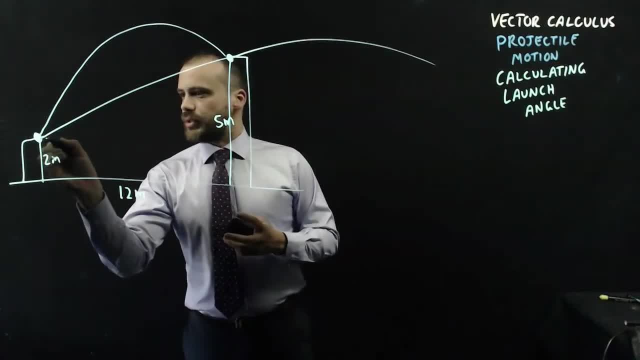 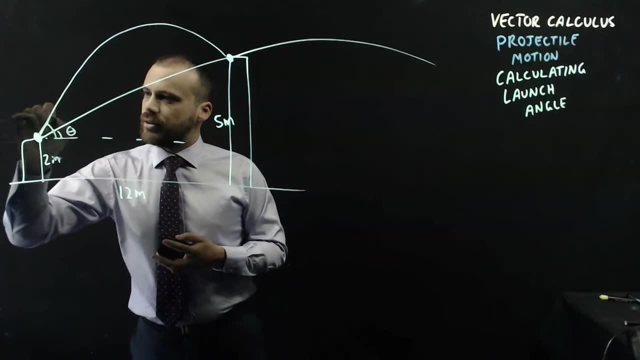 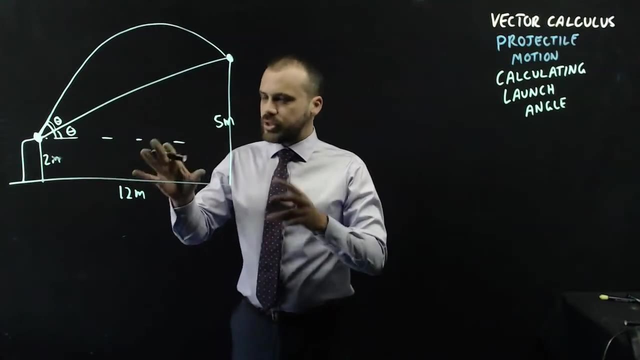 All right. so the question that I want is: what is the distance from here to here, What is that launch angle, or what is that launch angle? It's going to be two of them. Maybe not quite enough information here, because I'm also going to need to know if I don't know the angle. 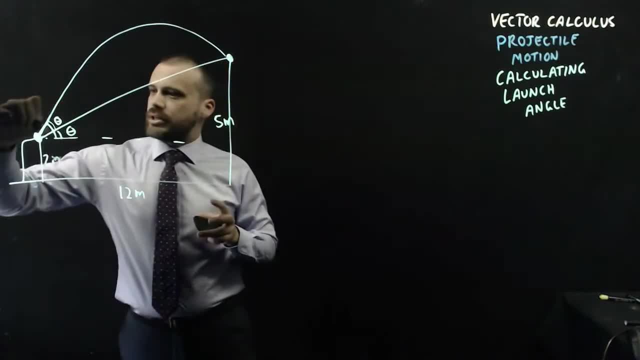 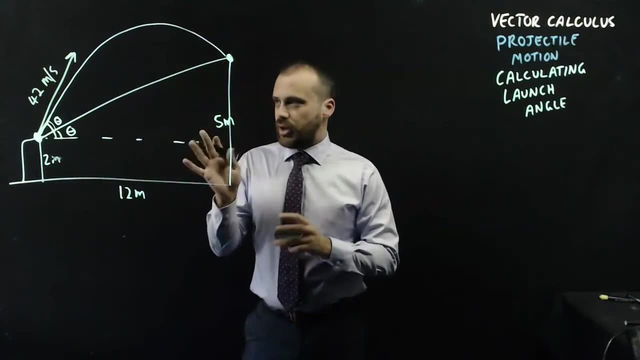 I at least need to know its initial velocity, All right, so let's give it an initial velocity of 42 meters per second. All right, that way we can start working with this now, because we have an initial velocity Now I don't really know. 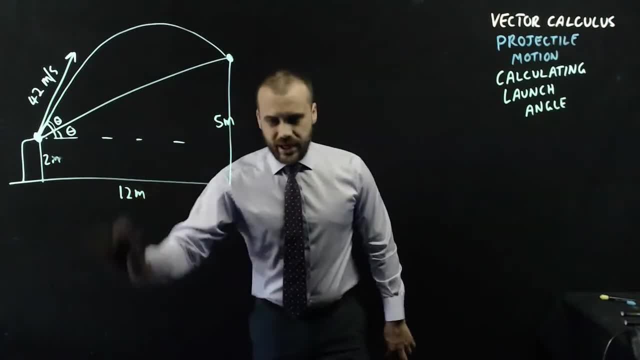 I don't know how to do it. I don't know how to do this question. I haven't tried it yet, but I'm going to do it here. Why don't we just write down our equations: acceleration, velocity, displacement. 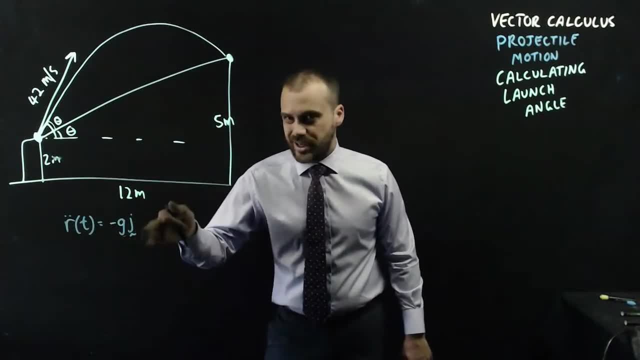 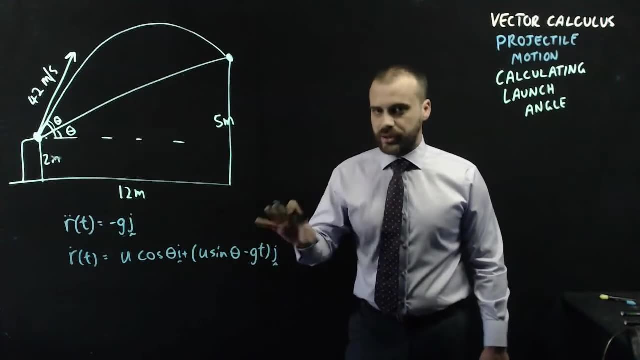 and see what they look like. Acceleration never changes. It's negative g in the j direction. Now this is our velocity function for any projectile. Now, if you don't know how to derive that, you probably need to go back and watch another video. 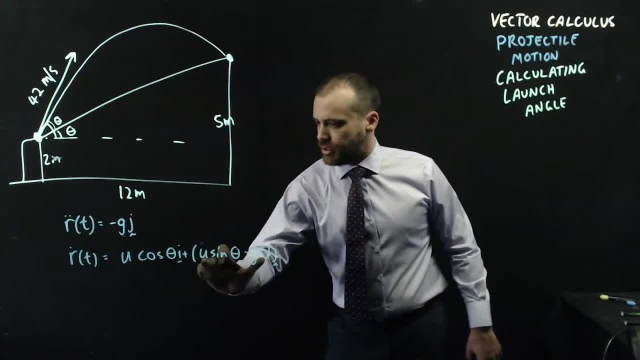 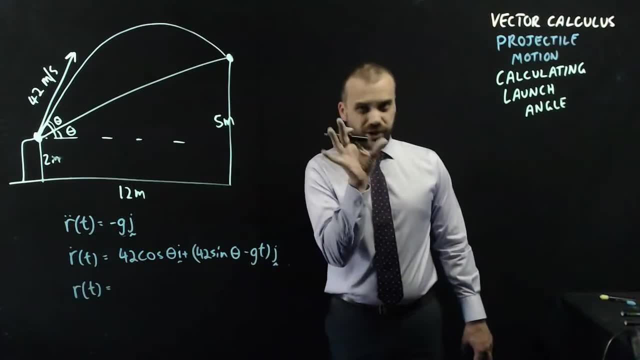 But these values here we know These are our initial velocities. so that's 42 and 42.. Now, finally, I probably want some sort of displacement function here. Now, before I do that, it's important to sort of get a frame of reference here, right. 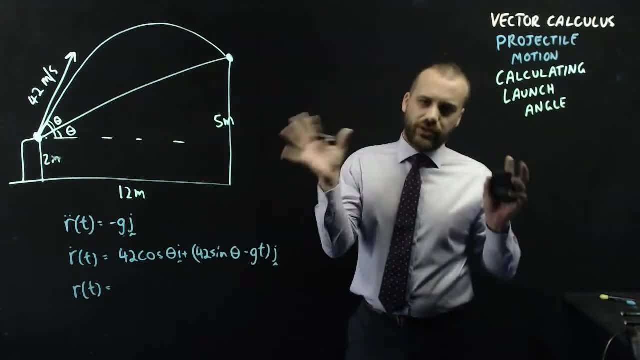 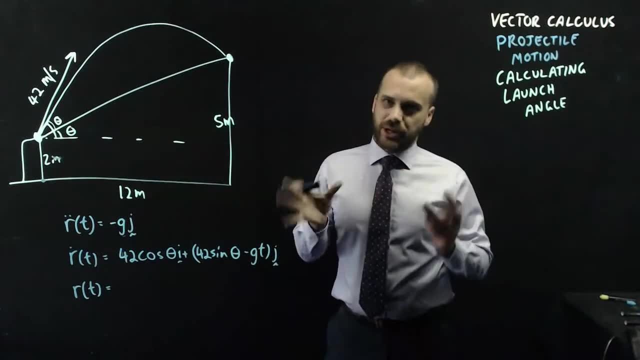 Because my displacement function is going to change depending on where I think my origin is- And some people might consider this to be their origin, but that's just going to lead us to a bunch of problems. Wherever possible, I'm going to create my origin where my projectile is. 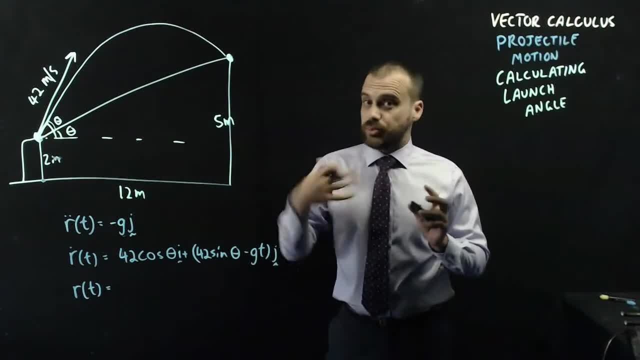 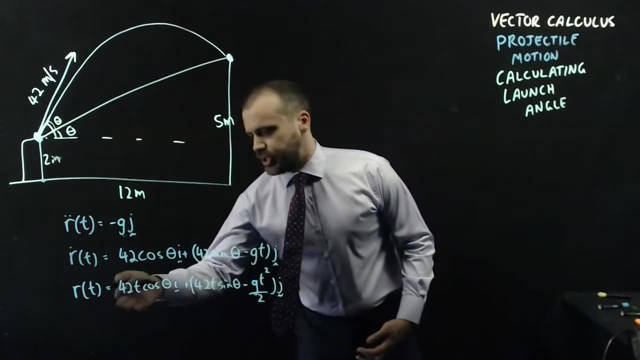 So that's going to be my 0, 0.. That means that its initial displacement is 0, 0, which means that I don't have to think too much about creating this displacement function. So I have my displacement function And this is really what's important. 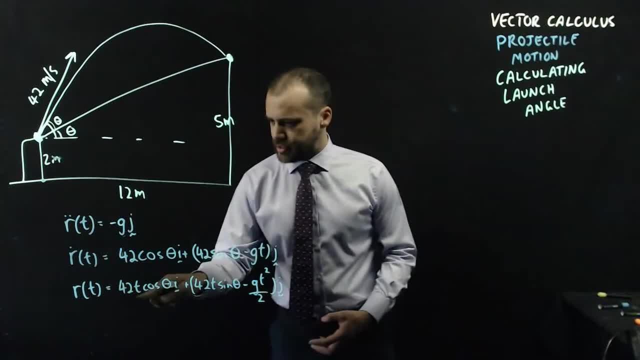 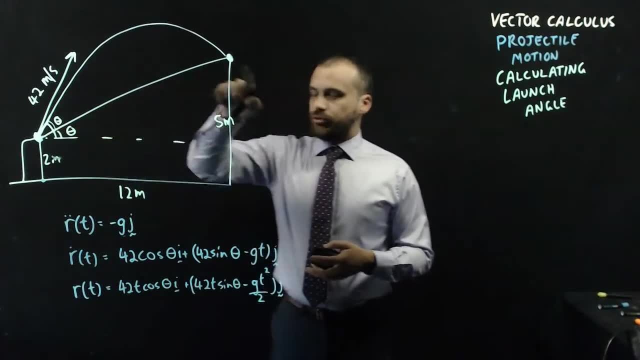 But this displacement function has a t value and a theta value there, So it kind of has two unknowns. Now I've got this quadratic or this quadratic. Both of them are going to be my answers at some point And they're both meeting at this point. 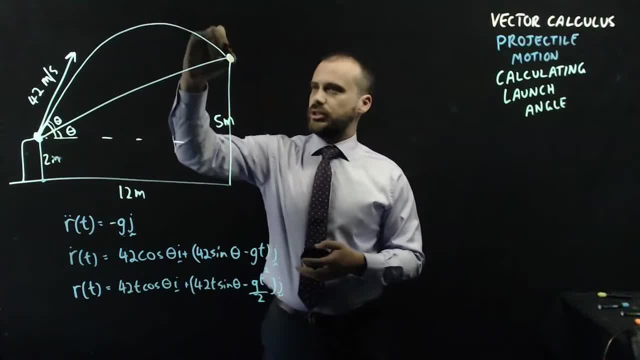 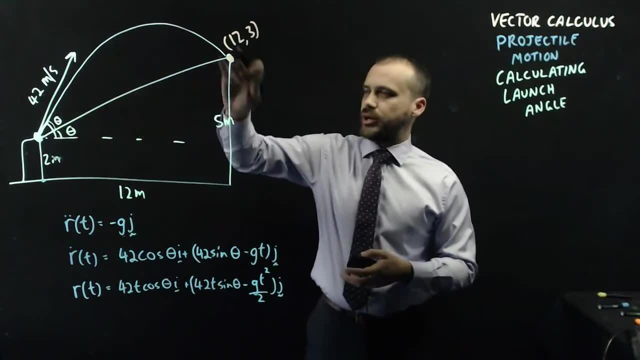 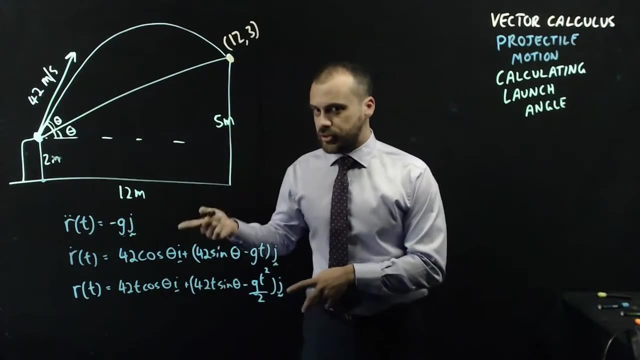 which- given I've decided that that's the origin- is actually coordinates 12, 3.. So what I have is a quadratic Passing through 0.12, 3.. If I could take this vector function and convert it to Cartesian form, 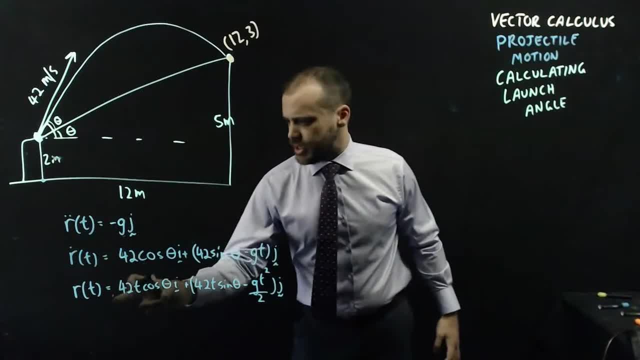 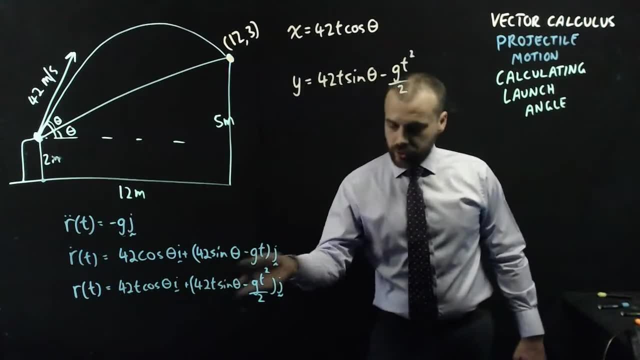 that's going to make my life way easier. So let's take this bit. My x coordinate at any given time is 42t cos theta. Let's take this bit. My y coordinate at any given time is 42t sine theta. minus gt, squared all over 2.. 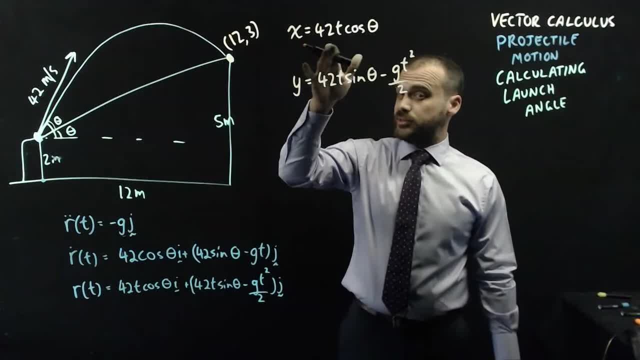 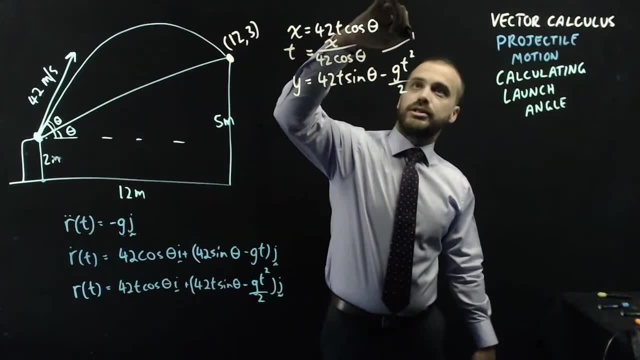 Now I just need to like set maybe this one to t. So if I divide both sides by 42 and cos theta, I get t equals x on 42 cos theta. I'll call this equation 1 and I'll call this equation 2.. 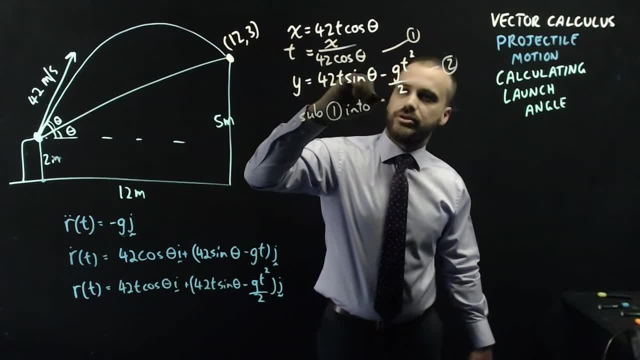 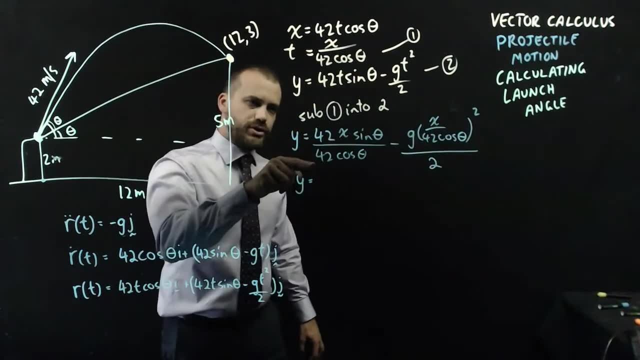 And now I'm going to sub 1 into 2 for t. Now, when I do that, I'll get this neat little thing here And you can see the 42s are going to cancel out. Sine theta over cos theta is tan theta. 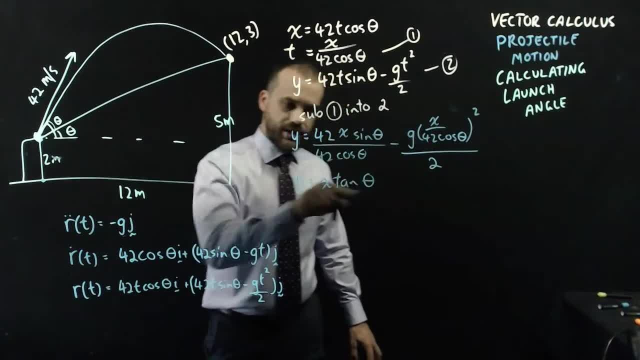 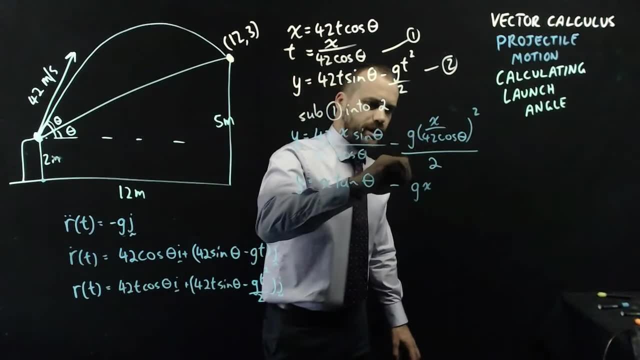 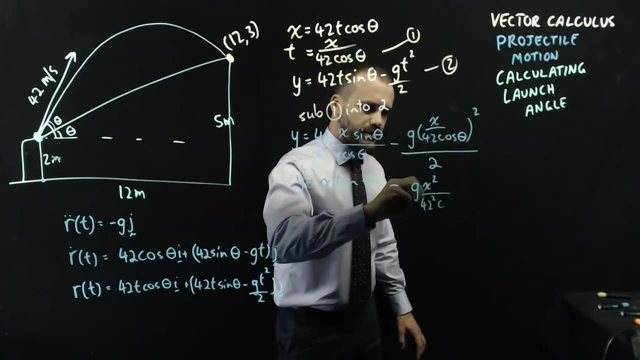 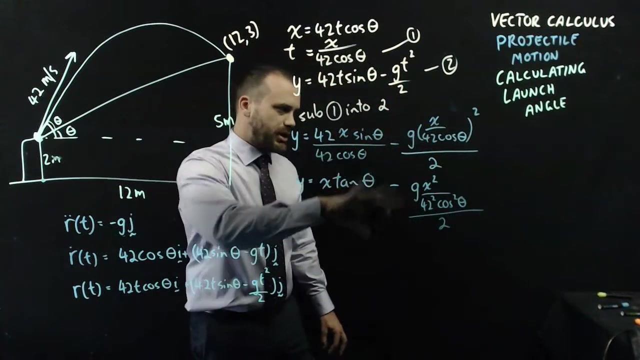 So I get this neat little x equals tan. Oh sorry, x tan theta. And then this little bit here: well, I get g. I get x squared over 42, squared cos squared theta all over 2.. Now I can tidy that up a little bit. 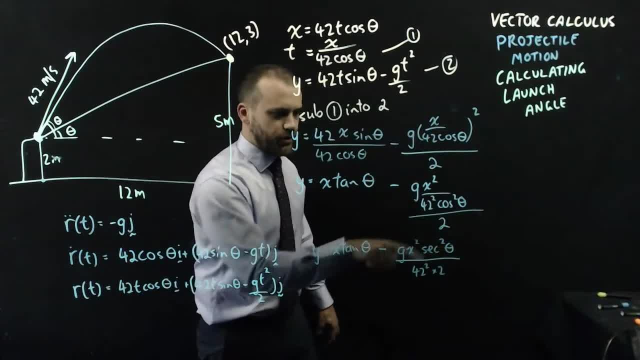 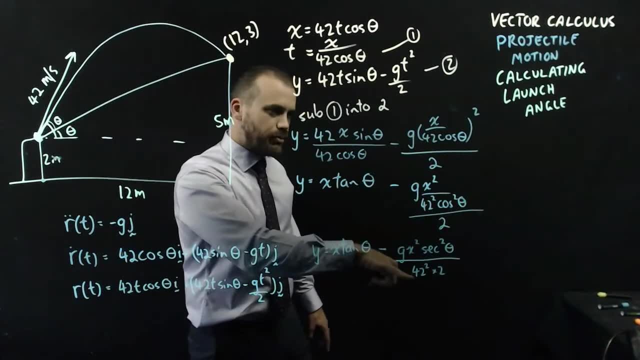 And we end up with gx squared 6 squared theta over 42 squared times 2.. Now just quickly. the 42 squared and the cos squared theta would both end up on the bottom of our fraction, But Over cos squared theta is the same as sec theta or sec squared theta. 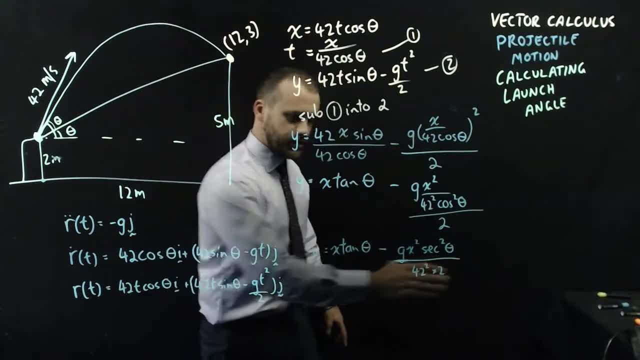 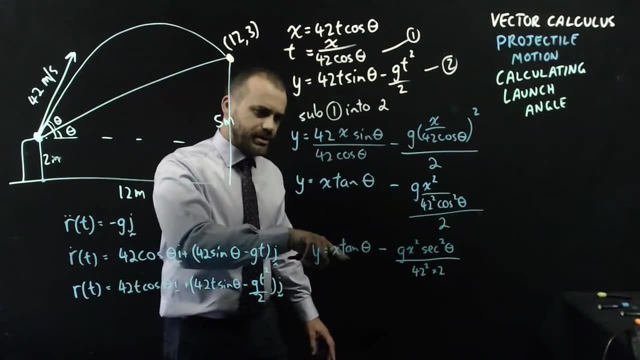 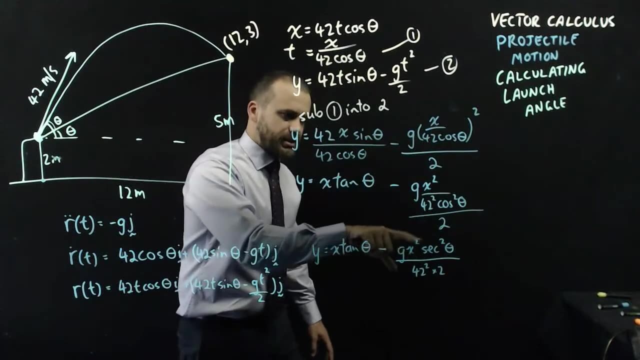 So just rewriting it like that, This is our quadratic. I know it doesn't look like a quadratic, but this is x, tan theta, right, And tan theta is just a number. if only we knew the launch angle. And this is x squared times a number, times a number over a number number. 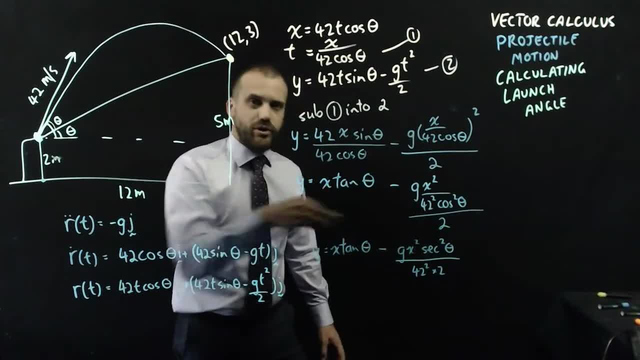 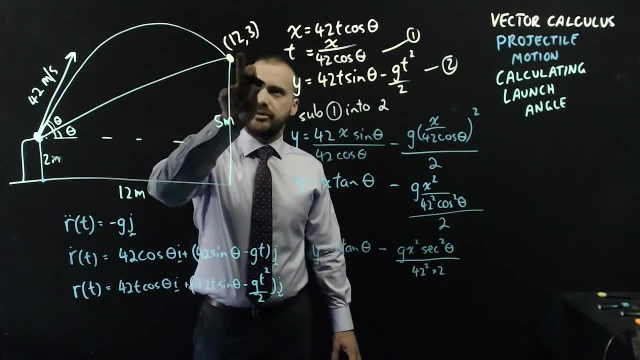 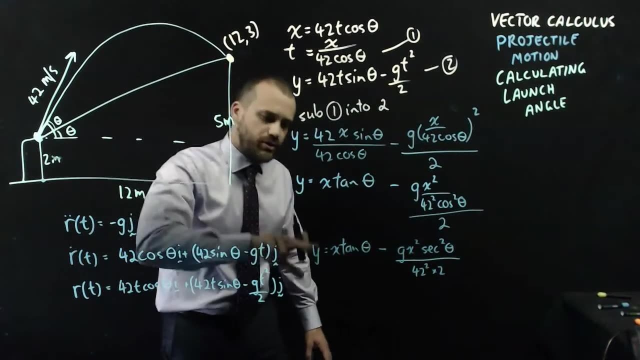 It's just x squared times a number. These are all numbers. If only we knew the launch angle. All right, so I have a quadratic. It's passing through point 12, 3.. I have the equation of the quadratic If I sub 12 and 3 in for x and y and solve that just using like an equation solver. 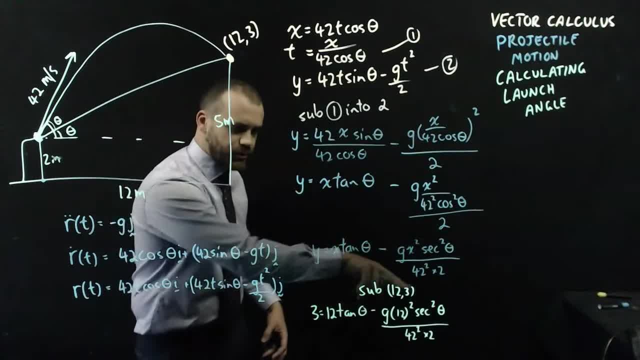 I should be able to solve it for theta. So here I'm doing that. I'm subbing 12, 3 in. You can see y is 3, 12.. Put another 12 in there: 12. 12 squared. 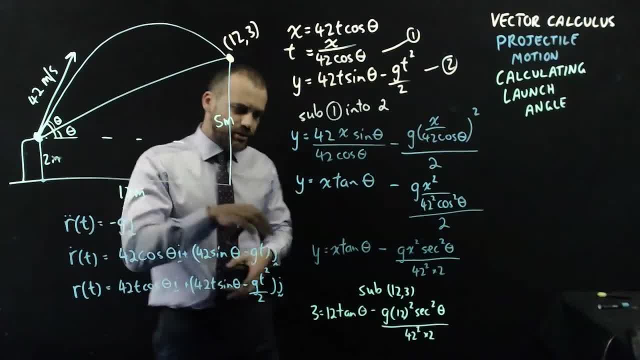 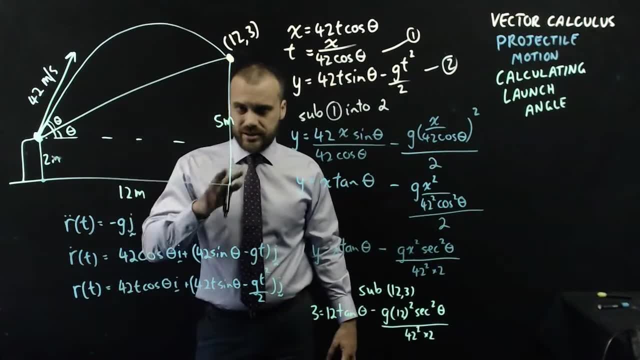 Now if I type that into my calculator, I can do it two ways. I can do like an: n solve Just type, n solve Type, all of that in and I'll get an answer. Well, I'll get a lot of answers. 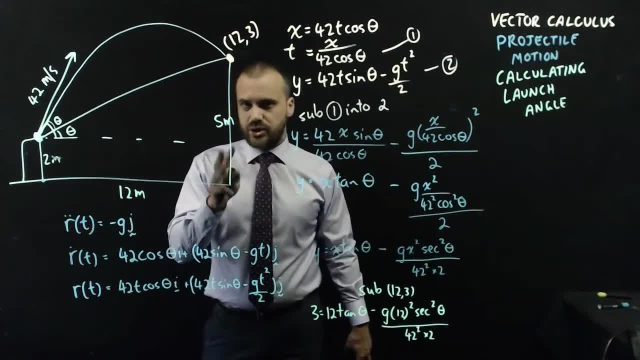 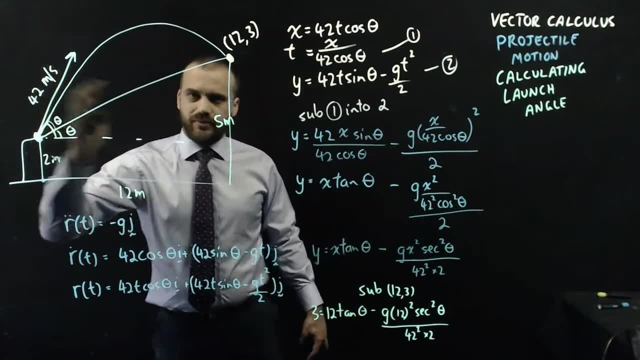 A lot of negative answers and a lot of positive answers. It would be up to me to interpret them and understand that. well, I need one positive answer and maybe another positive answer between 0 and 90. And when I type that into my calculator, I too get a lot of answers.